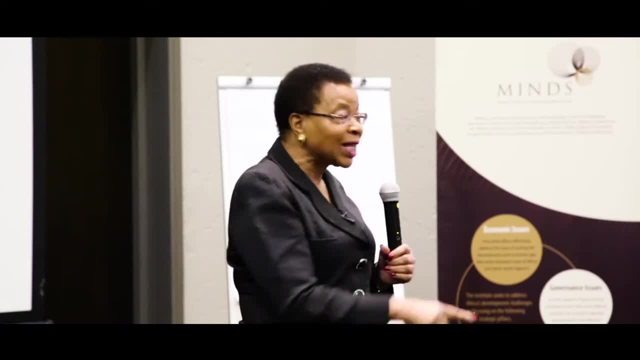 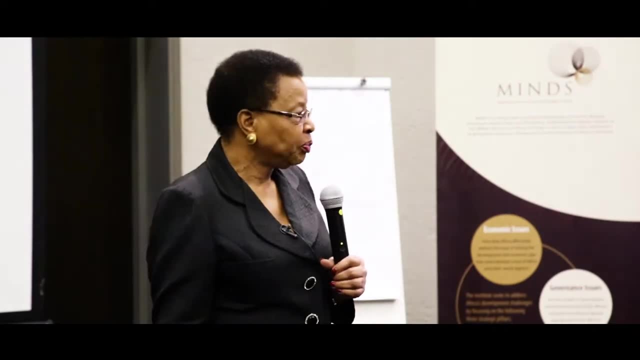 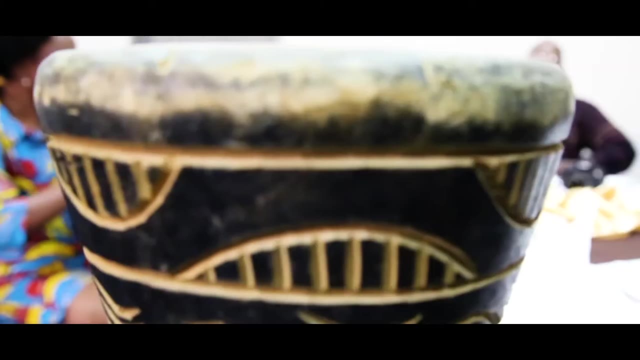 you as young people are going to produce as outcome of elections and those systems are going to govern your life, at least for the next 30, 40 years. What principle are you using for governance? I see an Africa with its own definition of democracy. 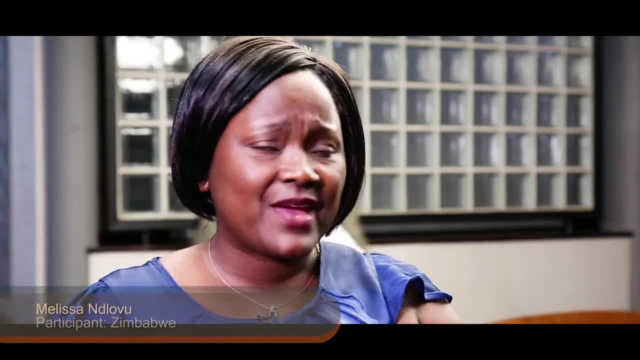 I see more open societies that respect the rule of law. I see strong institutions, both independent and state. I see more open societies that respect the rule of law. I see strong institutions, both independent and state. I see strong institutions, both independent and state. 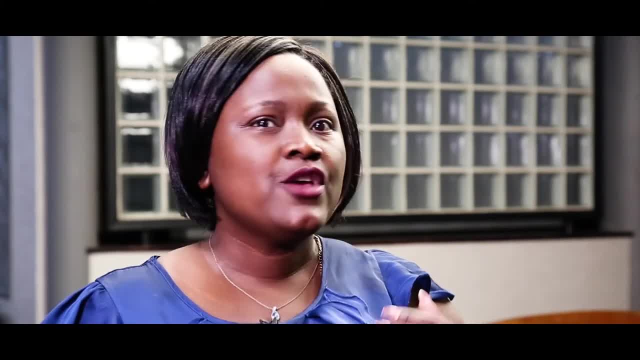 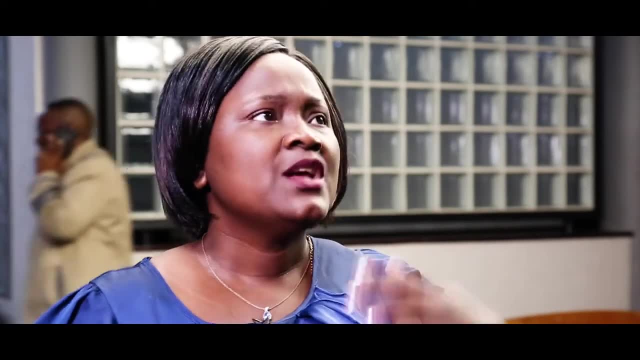 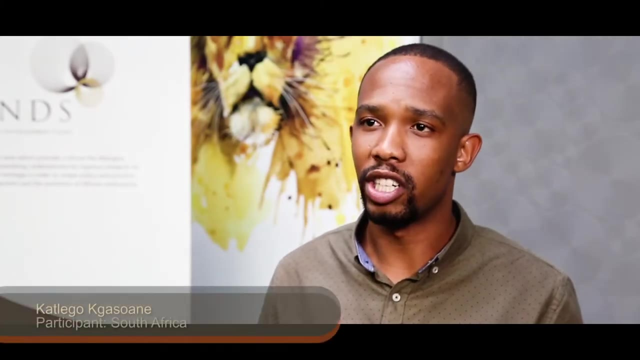 And state institutions that are able to respect the rule of law, human rights, protect the citizens rights and be able to allow communities and societies to articulate their issues, and having governments who are more responsive to their own societies. As the majority population here in Africa, I think we should be responsible enough to 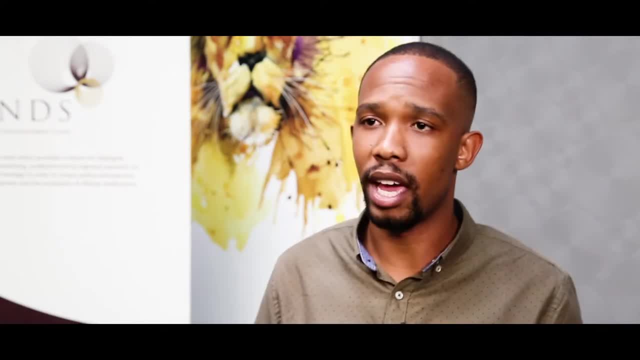 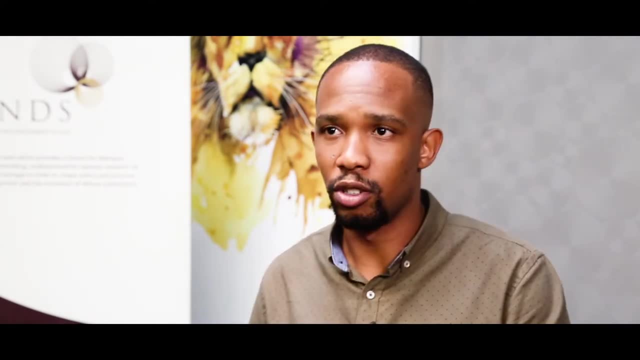 take ownership of the social issues that we have and by minds doing that, they are empowering us as young people to include. this is why we have it so richly valued. Yes, young people in Africa, They are assisting us, you know, through the workshop, through. 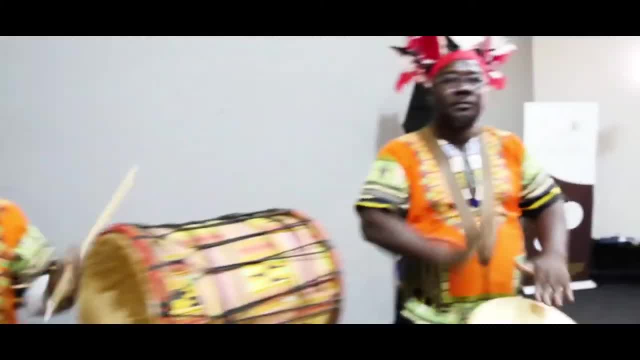 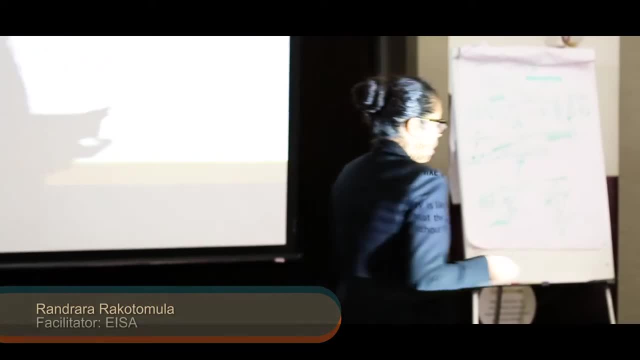 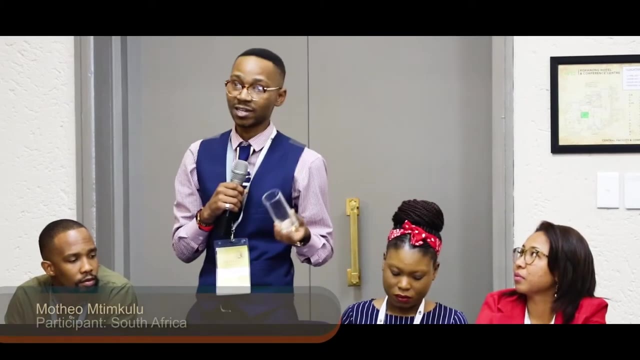 the youth dialogue that they have. We're engaging as young people and coming together to share ideas, A common understanding, a common definition of democracy. Democracy is like a glass: even when it's empty, it looks full. That's just to speak. 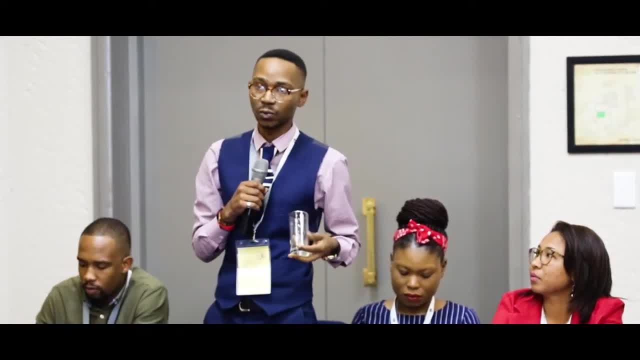 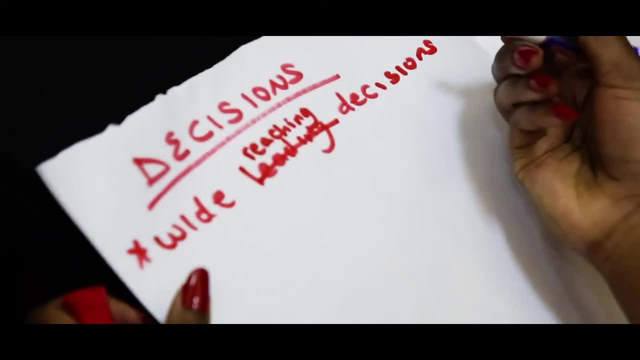 about that democracy is the best of all bad systems of governance. So you can't just say that democracy is benchmark and best system. It's just the best that we've actually figured out so far. When people are sitting around a table to do so, nobody around that table knows where. 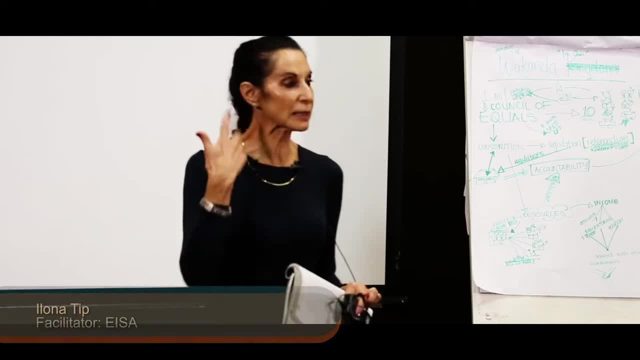 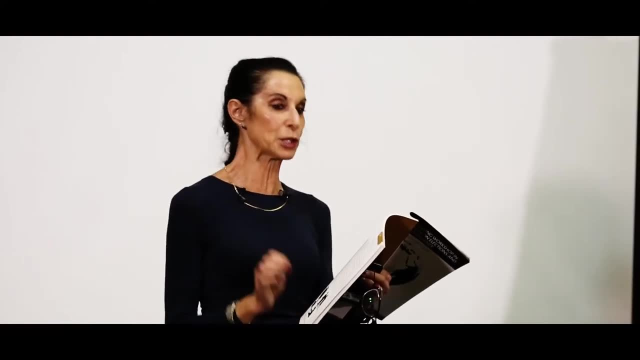 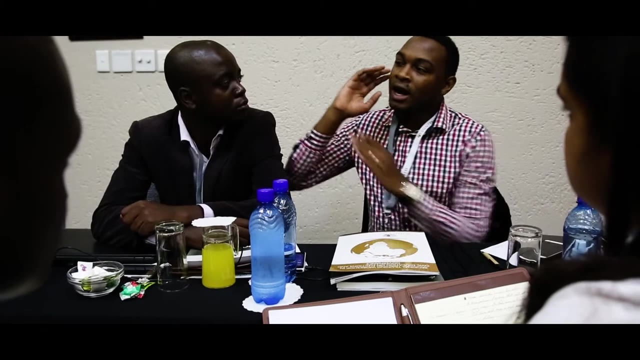 they're going to be in that system. So generally the thinking is that the most reasonable principles of justice are those everyone would accept and agree to from a fair position. We might say that's a bit utopian, because you mentioned Kama. people have ambition. 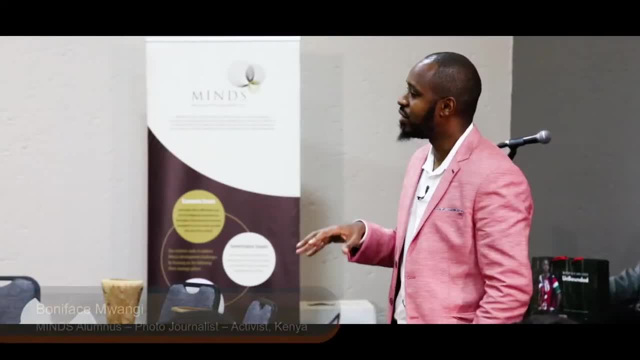 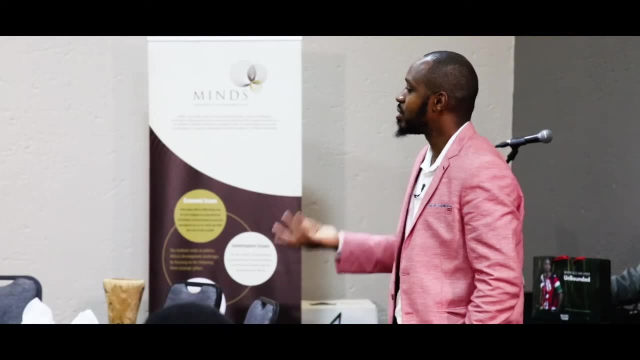 What do you do with them? The room can be full of slaves. They all hate you, they spit on you, but because your mind is liberated, you're still strong and you don't break. That's why they couldn't break Queenie. That's why they couldn't break Robert Subukwe. That's why they had to kill. 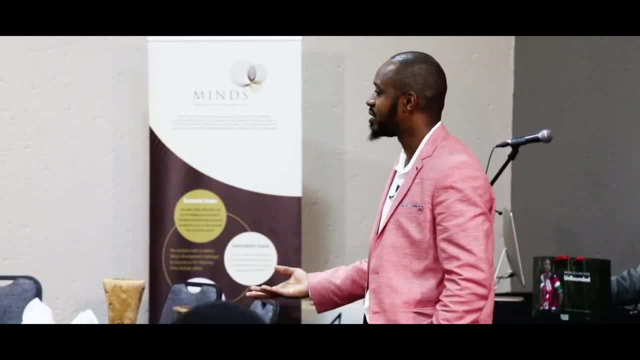 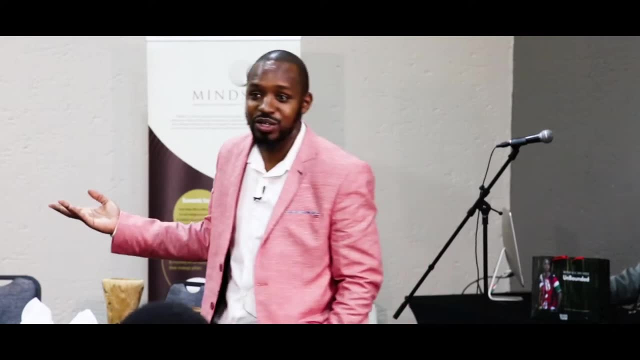 Chrisani before independence because they knew he was a threat to the system, And that is why some of you are going to get killed, perhaps, or you're going to get arrested or jailed, perhaps, Because the ideal and what you believe in 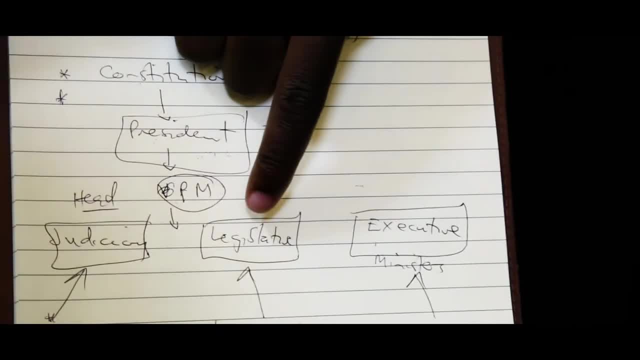 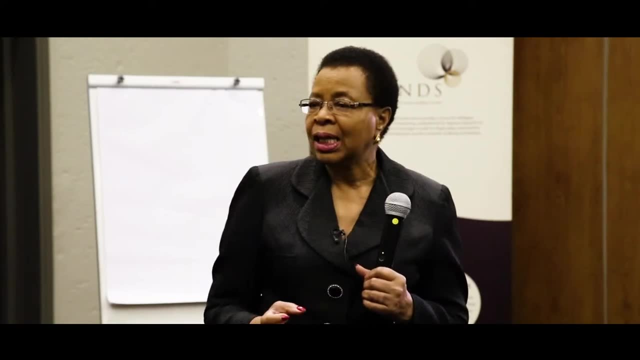 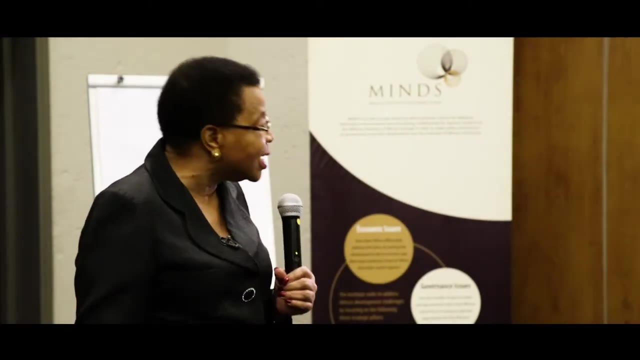 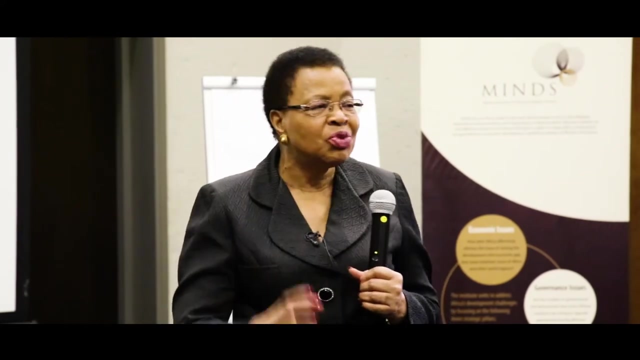 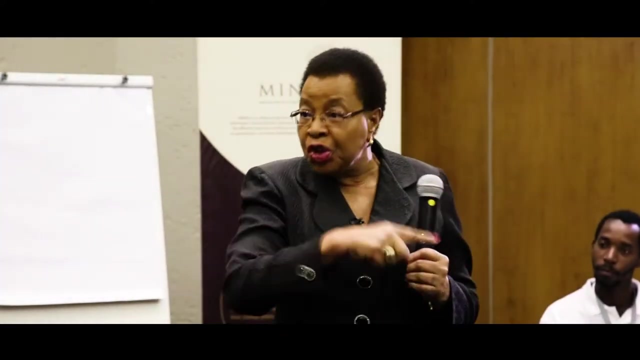 is bigger than yourself. You are perhaps, after the 50 years of our freedom, you are the generation who can stand and decide what kind of electoral systems we want, In other terms, what kinds of elections we want: democratic systems. we want to serve you, to serve your children and grandchildren. 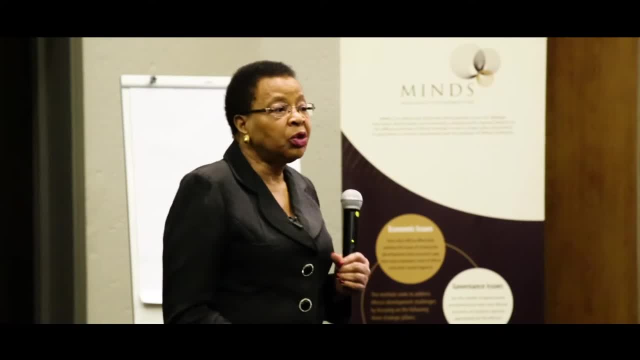 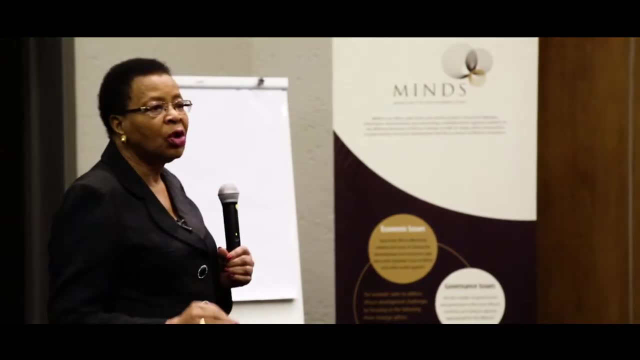 And if it is important for you, if you feel that we have to turn the tables around of what exists as electoral systems, who can stop you from doing it? It just showed me that some countries tick all the boxes, but you really have to look. 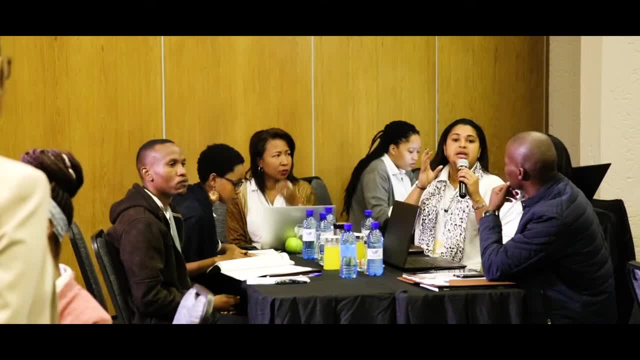 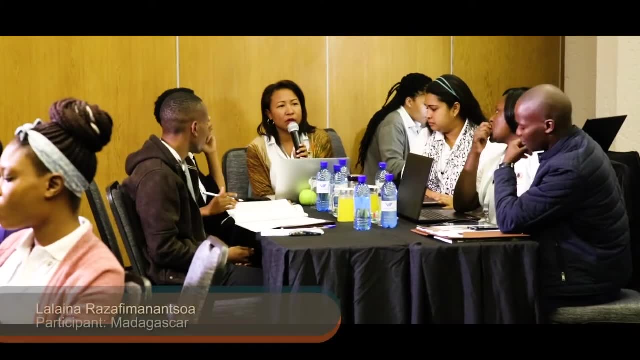 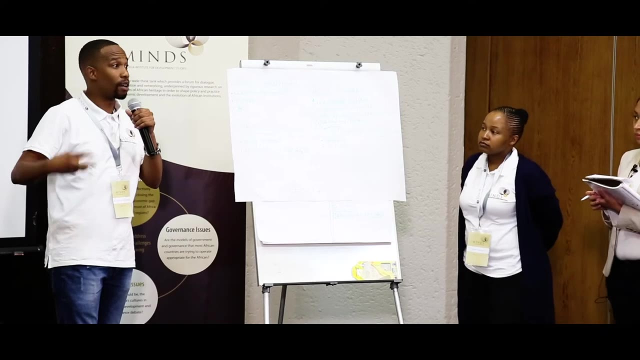 in depth to find out whether they really really are practicing transparent and democratic practices. Just to add, we have also looked at the electoral cycle, which is very important, because election is not just the period that we go to vote, but there is the pre, there is the post and 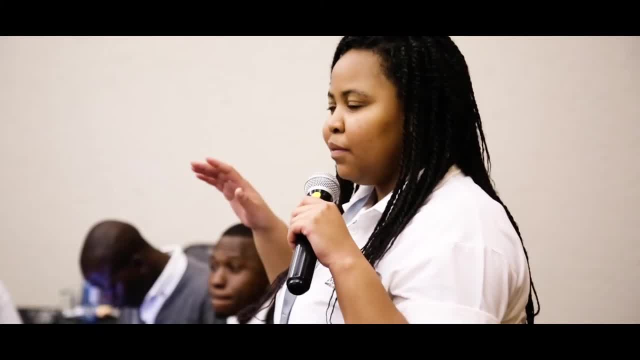 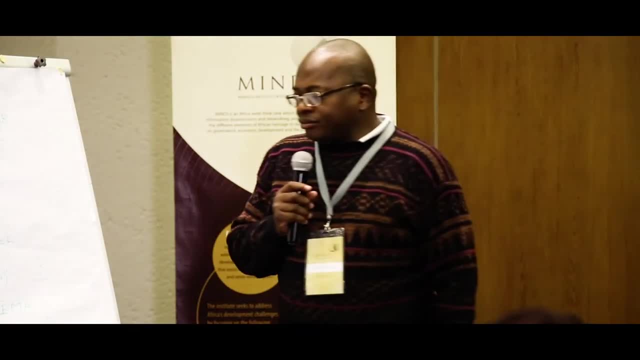 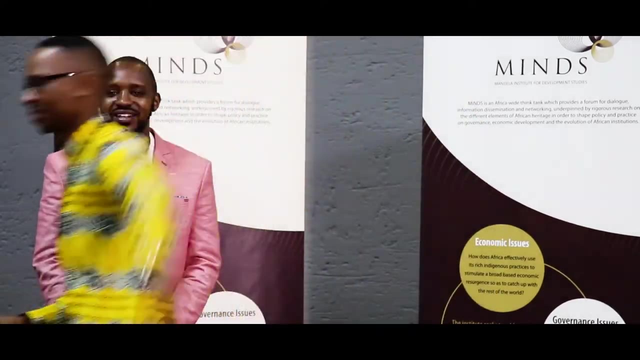 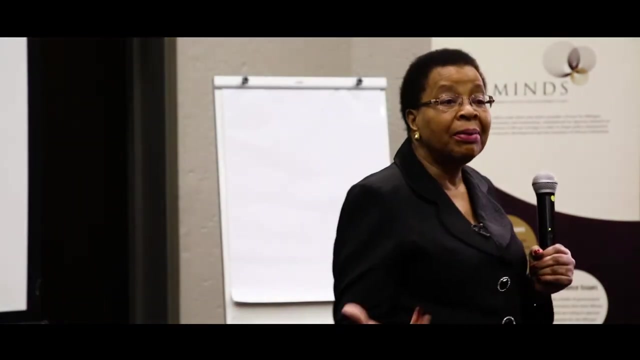 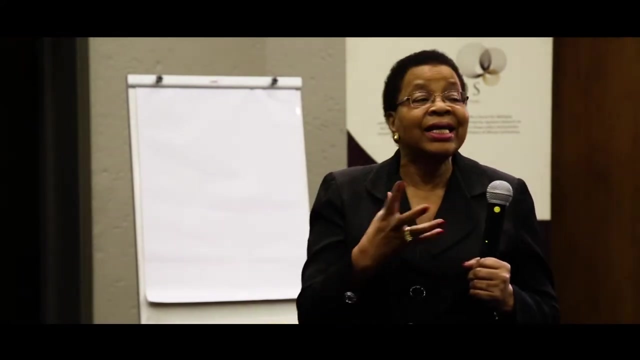 all of those phases are very important to ensure accountability, transparency and inclusive process as well. Let me say why this is so important. All the other, the so-called developed world, the developed world, whether it's in Asia, whether it's in Europe, whether it's in America, they have systems which you today, you clearly 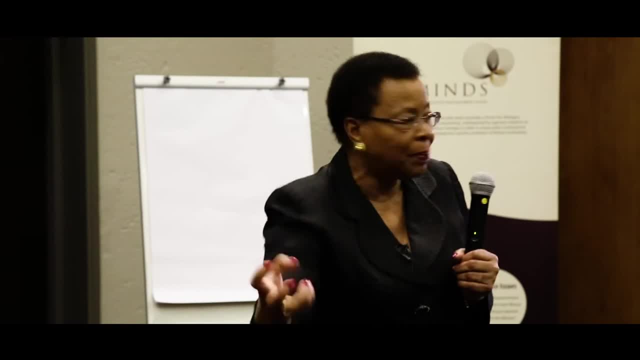 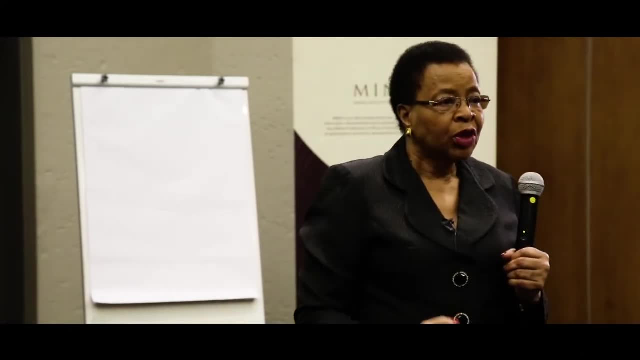 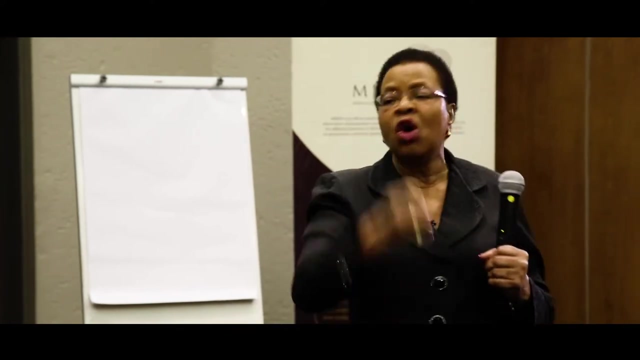 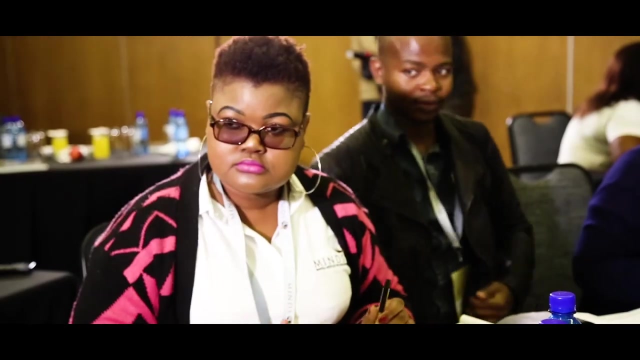 identify that this is American, this is Japanese, this is German, this is French, this is okay, this is American, This is French, Okay. So can I ask you, what can you say that this is genuinely African system of governance? 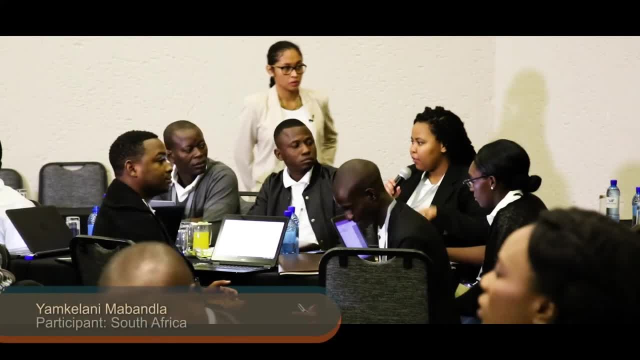 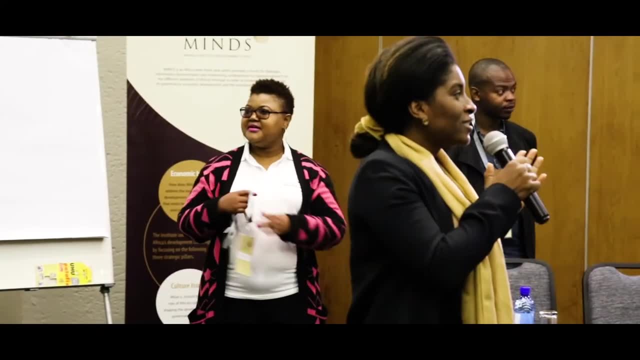 Something else that was quite important from yesterday- I think happened before the sessions, when we were speaking about the different expectations we had. so I think as we go along, we can keep checking to see what we've achieved and all the other things we still have to do. 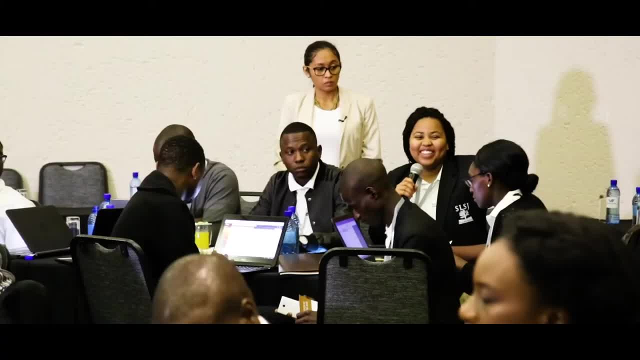 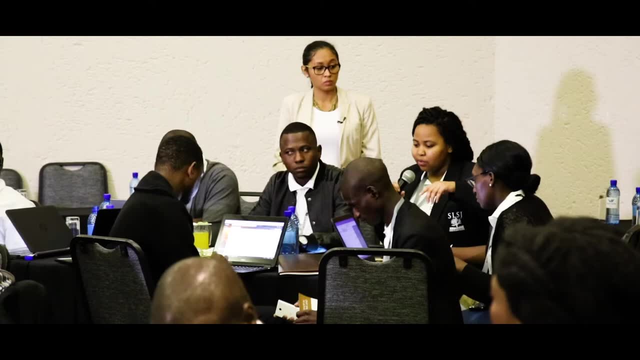 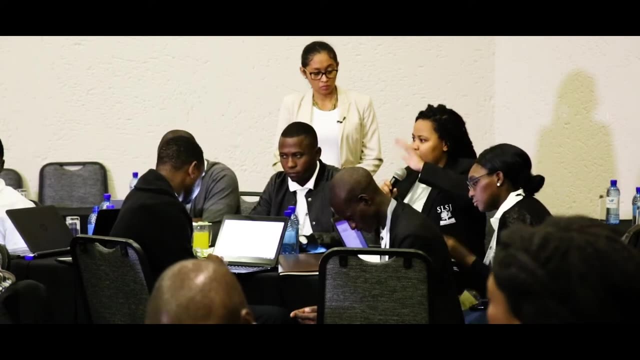 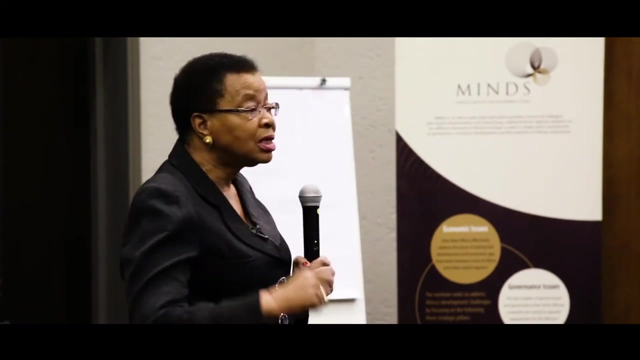 And all the expectations are on the wall if anyone wants to read them. But I remember one of the ones I had mentioned was particularly learning how to structure and affect meaningful African collaboration. You will be the first generation of Africans to shape what are the systems which work for. 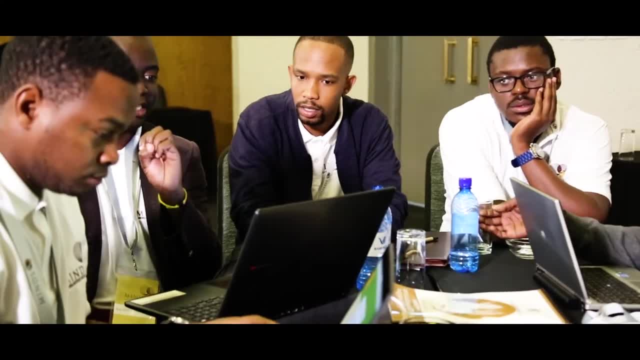 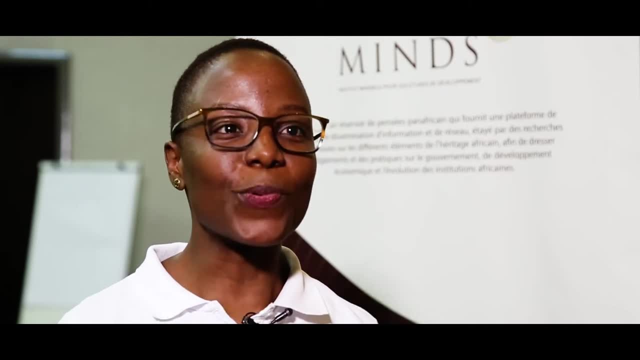 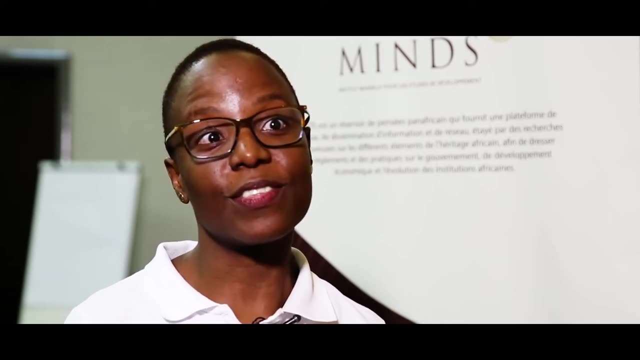 Africans and for Africa. Thank you, Thank you, Thanks, Thanks. We were definitely impressed by the caliber of the participants even before they came to the workshop, So we went through a very thorough screening process. We received over a thousand applications and only narrowed it down to 30 people who could. 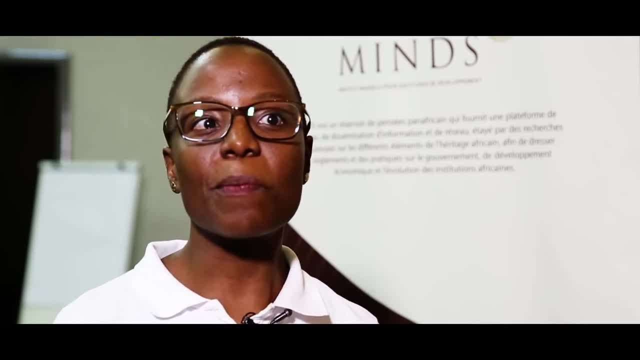 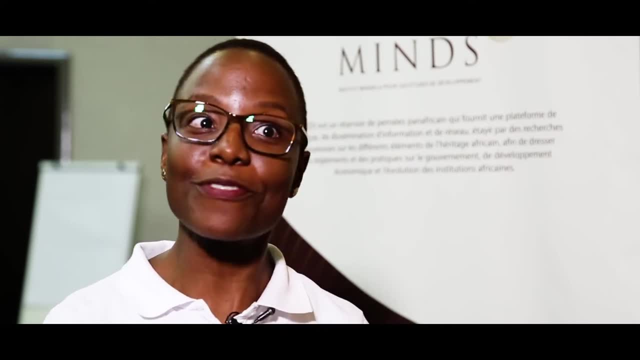 attend. So it was a very tough job for us to pick the 30, but we felt that we did a really good job to identify the right people that needed to be there with us. So they were impressive even before they showed up. 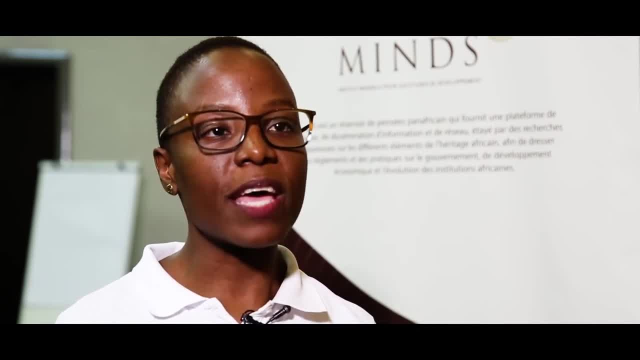 But having gone through the two days, we were told that we would have a really good job. going through the two-day journey with them, we have even greater faith that they will take the work, they will take the message, they will take the challenge that Mrs Mashal put to them and 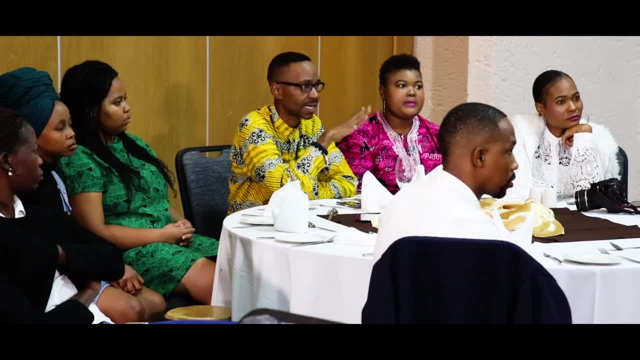 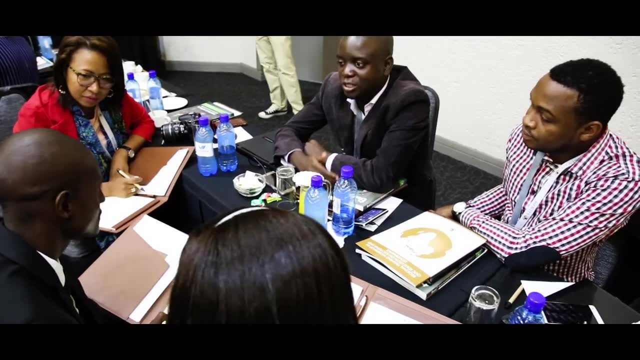 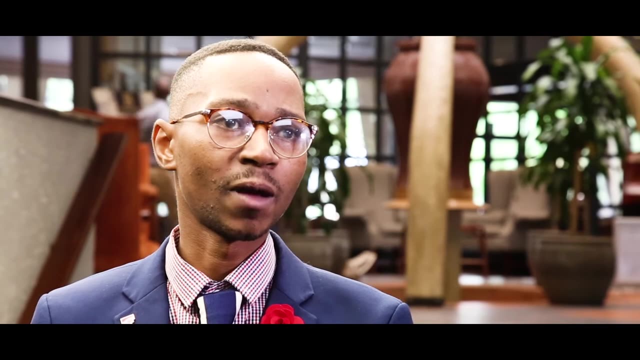 they will take the charge to lead other young African individuals to participate in elections and governance. You know I've intimated to some of my fellow delegates that the ultimate goal is the presidency, so hopefully MINDS is one step closer to that understanding intimately. 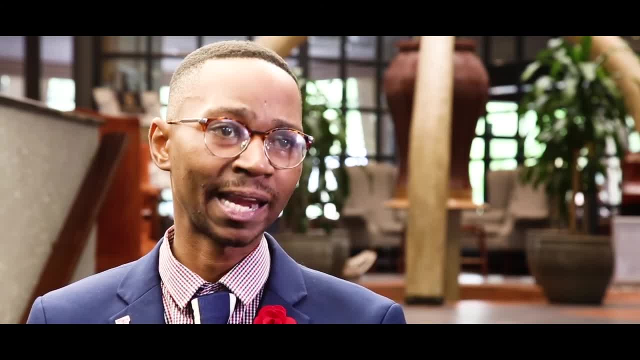 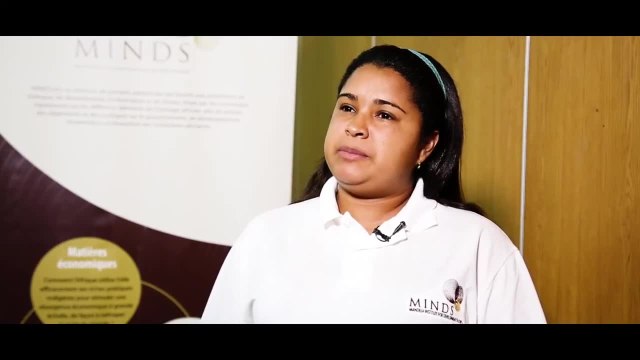 what elections are about. having been on the other end getting people's votes, it's going to be very interesting to understand how the business of elections works. The best thing about this program is that it brings people from different countries together and you're able to sit in. 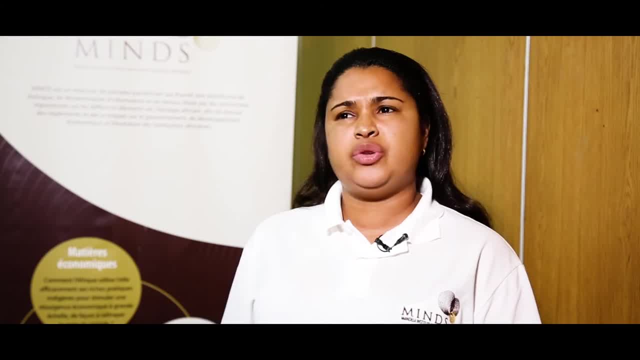 a room and hear other people explain how it works in their country and how it's not working in their country. so you get the best practices and at the same time you hear of the best coming from different countries that have come to see this, and hopefully that goes with thenegogeةorg. 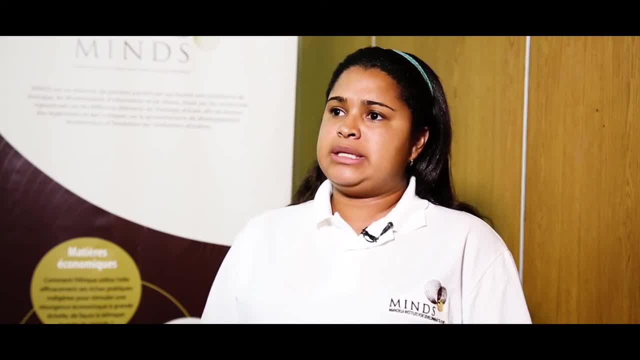 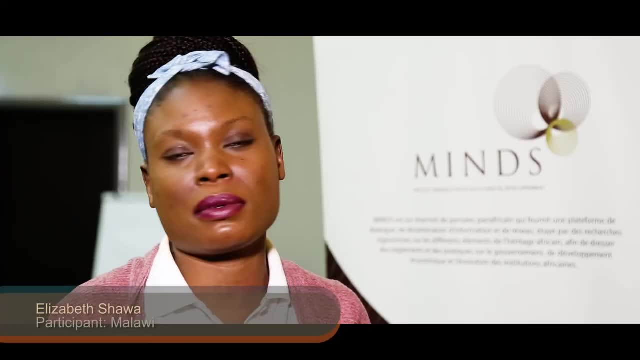 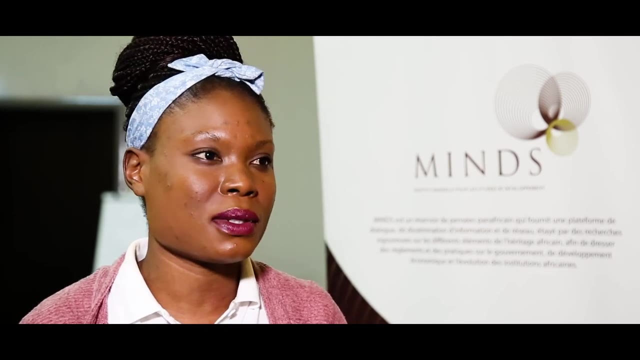 issues and difficulties that they're facing. so, in a way, it, it, it. it permits you to appreciate what's happening in other countries as well as your own. I mean having to meet with different people from different countries and you hear them having sharing their experiences. for me, that was it feel it.